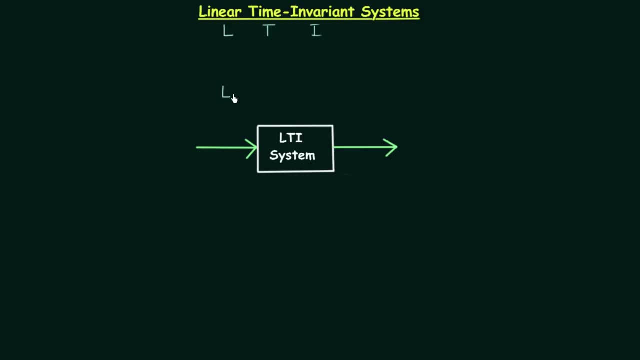 And the second one is time invariant system. The first one is linear system And the second one is time invariant system, And because of this only we call it linear time invariant system. It is combination of linear and time invariant systems And therefore LTI system will. 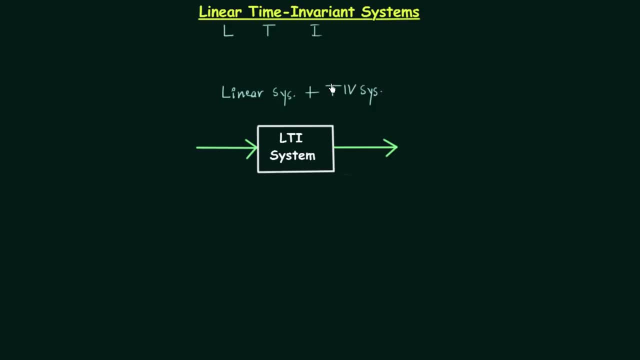 possess the properties of both linear and time invariant systems. We already know the linear systems follow the principle of superposition, So the LTI system will also follow will also follow the principle of superposition, superposition, position. This means the LTI system will satisfy both the law of relativity and the law of 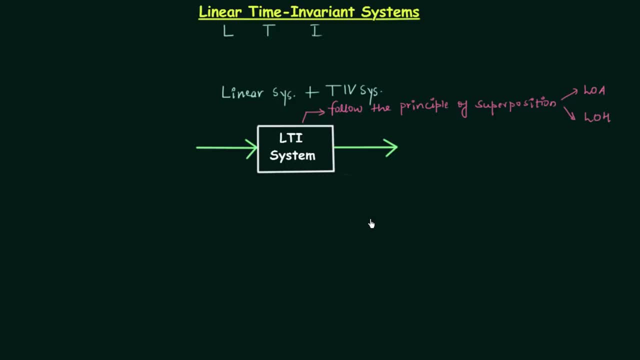 homogeneity. Now time. invariant systems are those systems in which any delay in input is also reflected in the output. So the LTI system will have the output, in which the any delay in the input is reflected. any delay in the input is reflected in the output. so the LTI system will possess the two. 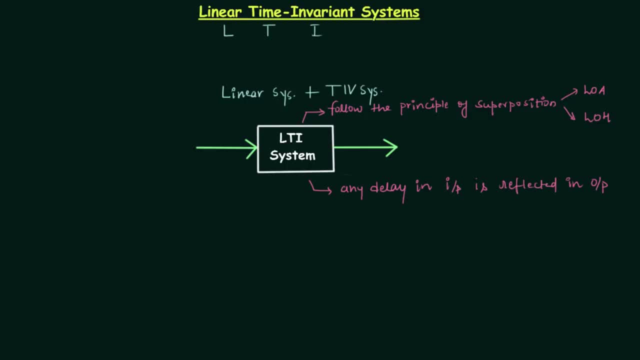 properties which you can see on your screen, and like usual notation which we are following till now, the input will be represented by XT and the output will be represented by YT. now there is one important parameter known as impulse response. the impulse response means the output of the LTI system when the input 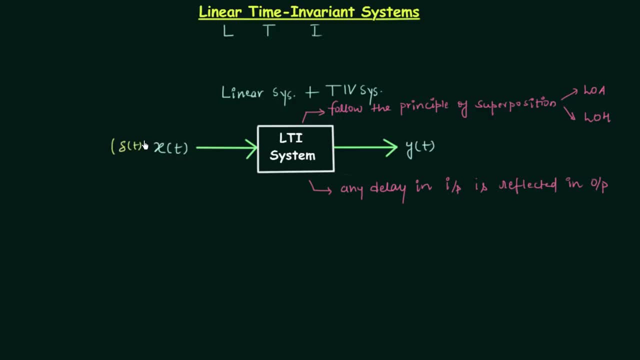 is an impulse. XT is Delta t. the impulse and then the output of the system for Delta t is known as impulse response HT. this is the representation of impulse response and the impulse response is used to define a loop. the LTI system. The impulse response is very important parameter. It is used to define the 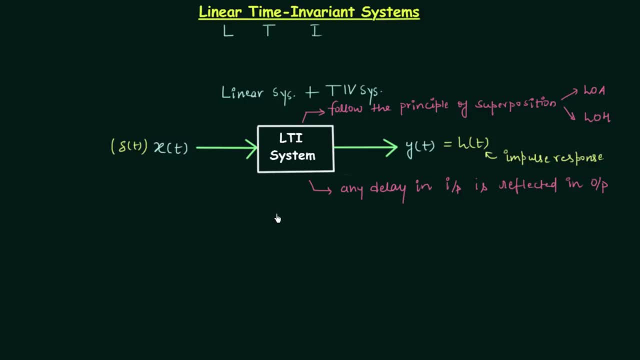 LTI system and the transfer function is also used to define the LTI system. The impulse response is in time domain: Xt, delta, t, yt, ht. everything written here is in time domain. But if you want to calculate the impulse response using the system relationship, the relationship between output and 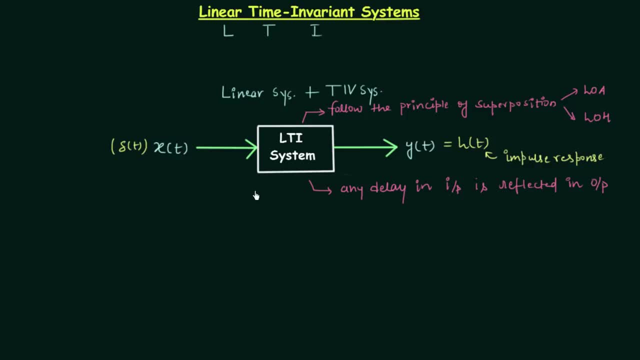 input, then it will be difficult in time domain. That's why we go to the frequency domain using the Laplace transform. You can also use the Fourier transform, But in this chapter we will mainly use Laplace transform. So by using the Laplace transform we go to the frequency domain. 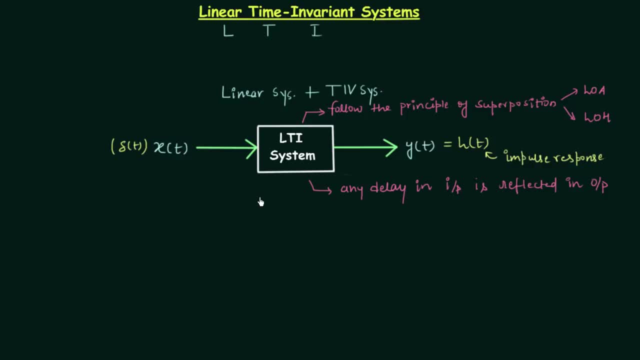 you will have the system relationship in frequency domain And by using that relationship you can calculate the transfer function. So our LTI system is defined using the impulse response input. But impulse response is not given. the relationship between yt and xt is given, So we will go to the 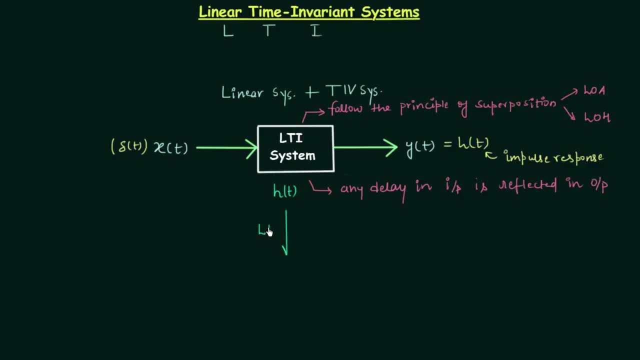 frequency domain using the Laplace transform or using the Fourier transform, And by doing this we can easily calculate the transfer function h, omega or hs. By using the Laplace transform, you will get hs And by using the Fourier transform, you will get hs. 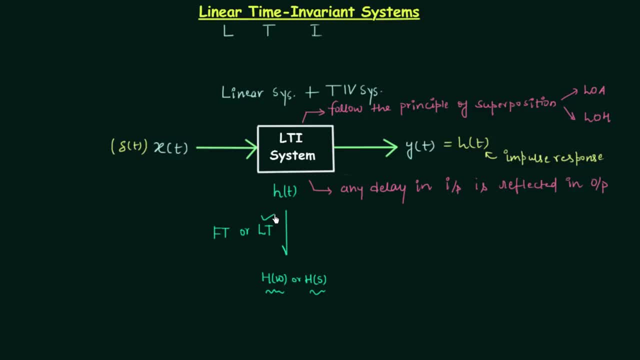 by using about h omega. in this chapter we will mainly focus on Laplace transform, So our transfer function will be hs. And now you want the impulse response. you had the relationship between output and input, you used the Laplace transform to obtain the transfer function, and now you want to go back. 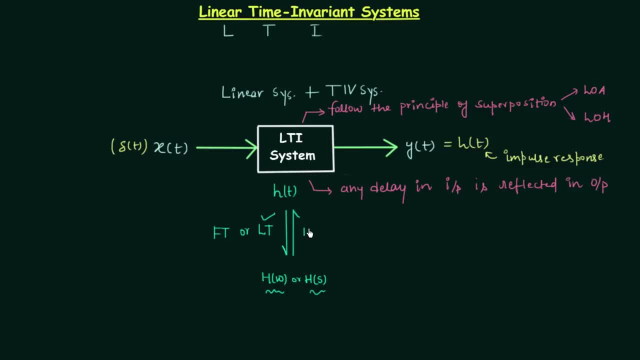 to the time domain and you can use the inverse Fourier transform or the inverse Laplace transform It. it will give you the impulse response. and now we can easily comment about the other properties of LTI system. So impulse response and transfer function: both are used to define the LTI system and 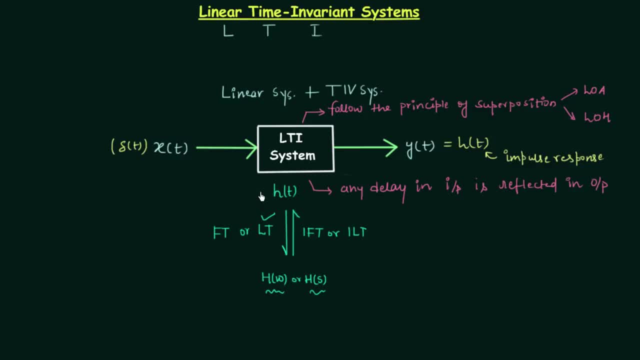 if you have any one of them, if you have the impulse response or you have the transfer function, you can comment about the other properties of LTI system. Now there is one important point which you should remember: the impulse response and the transfer function are only used for LTI systems. 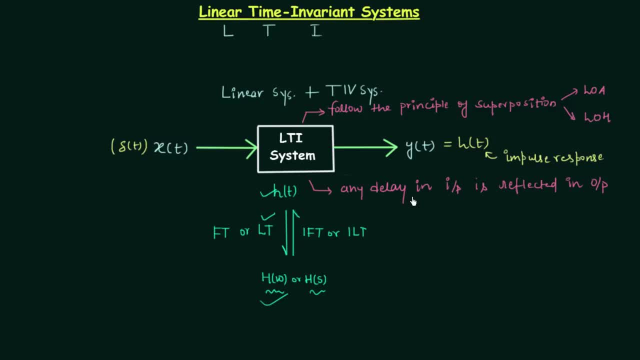 If we have a non LTI system, then we cannot have the transfer function or impulse response for that particular system. In the next lecture I will explain the process to calculate the transfer function, I will explain what is a transfer function and I will take few examples to make you understand.